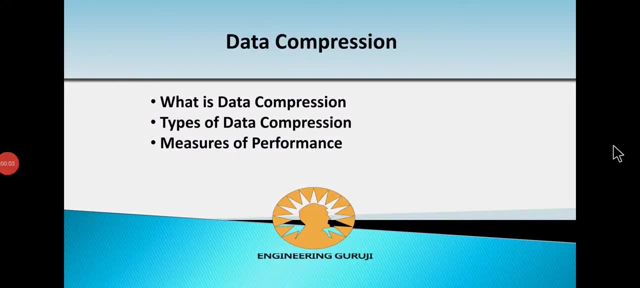 Hello students, Today I am going to discuss introduction to data compression. In this video lecture, I will discuss what is data compression, what are different types of data compression and what are the measures of performance of different data compression techniques. Let's start. what is data compression? 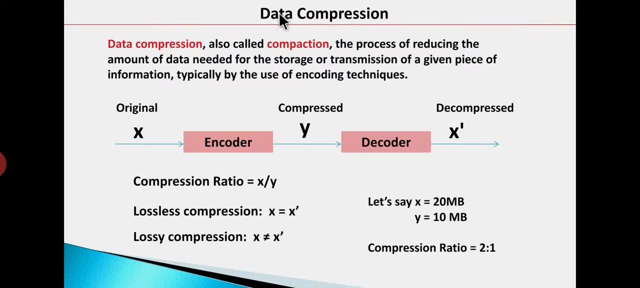 Data compression consists of two words: data and compression. It means we have to compress the data. okay, So data compression is also called as compression. So what is the definition? The data compression is the process of reducing the amount of data needed for the storage or transmission of a given. 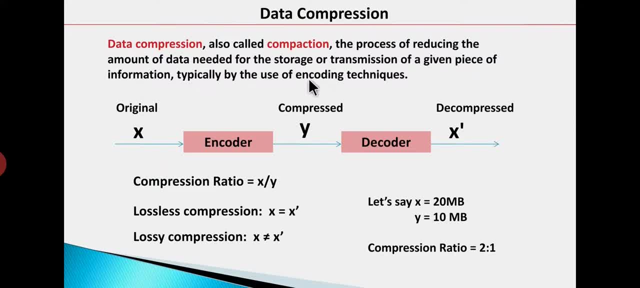 piece of information, typically by the use of encoding techniques. So data compression is a process through which we reduce the size of the data so that the memory used to store it decreases And we can easily and quickly transmit it. okay, And for this we use encoding. 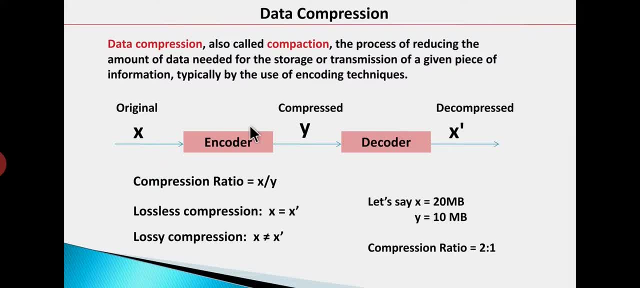 techniques, okay. So let's see the figure. This is X is your original data. and now here is an encoder. is there? It is used for encoding, okay? And this encoder will compress the data X. So data X after compression becomes Y. Y is the compressed data. 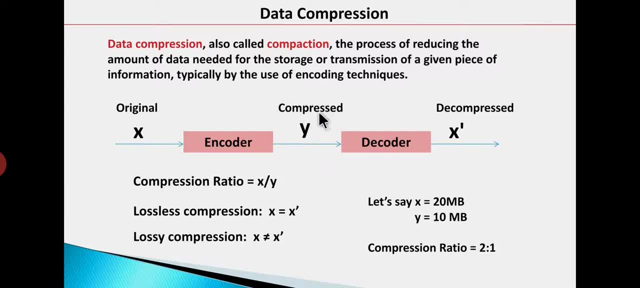 Okay. Now if you want to convert this compressed data back to the original data, then we have to use decoder Means decoding. So if Y is decoded by a decoder, we get X dash. So what is X dash? This is the decompressed data. X is your original data, Y is your compressed data. 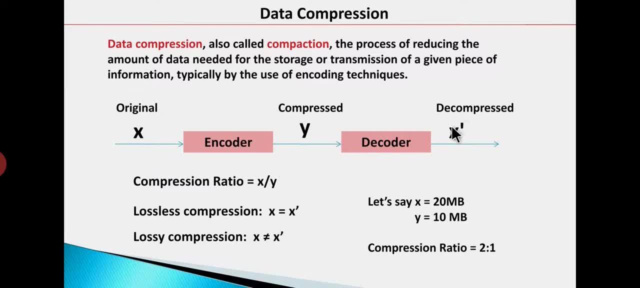 after encoding: And X dash is your decompressed data after decoding. Okay, Now lets see that if X, Which is our original data, And after decoder, if X dash is being received, So if X dash and X are the same Means, after decoding we get our 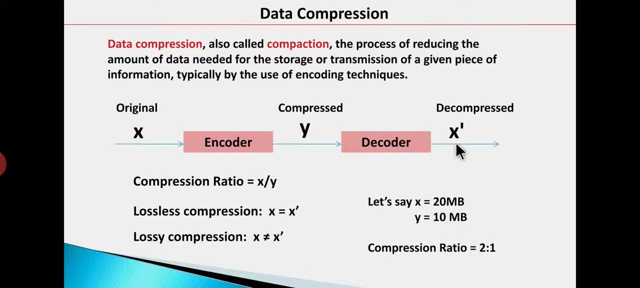 original data. X. Okay, It means there is no loss of data. So what is here? X, which was originally original, That X in a certain way is getting decomorphized again. This means that in your data if you have X, then Y is decompressed and the X is also decomposed in the same way. 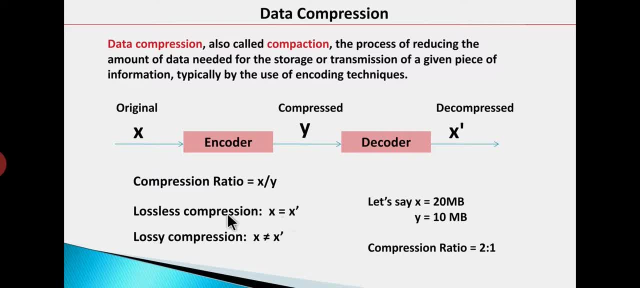 loss is not happening. So this type of compression is called lossless compression, Where the original x is same as x dash, which is we got after decoding, And if there is some loss of data, if there is some loss of data, then x and x dash will not be equal, because there 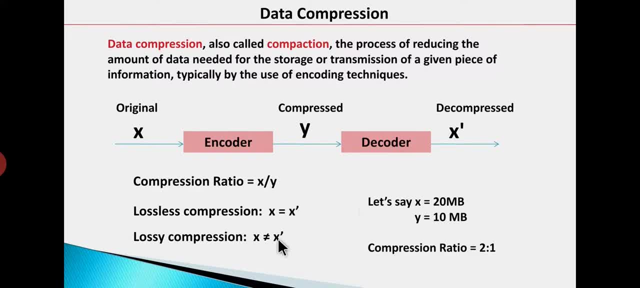 is some loss of data after decoding. So if x is not same as x, dash, it means the compression is called lossy compression. So in lossless compression there is no loss of data And in lossy compression there is some loss of data Means the x which is original. we don't. 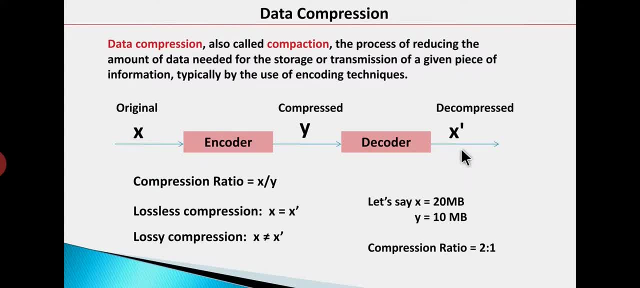 receive the same x here. Okay, Because of some loss. Okay, So data compression techniques are basically of two types. One is lossless compression, in which there is no loss of data, And the other is lossy compression, in which there is some loss of data. Okay, Now we 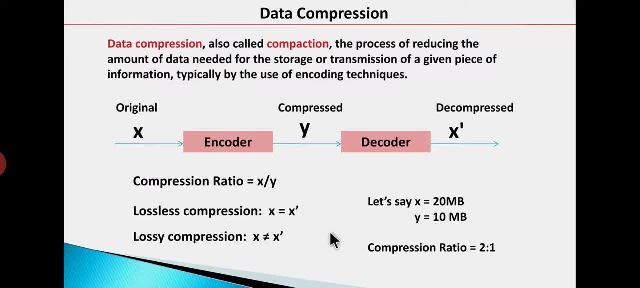 will talk about how much data has been compressed. Okay, So how we measure this? This is measured by compression ratio And this is defined by x, by y. x is your original data and y is your compression data. Okay, For example, if x is 20 MB, Okay, And after compression? 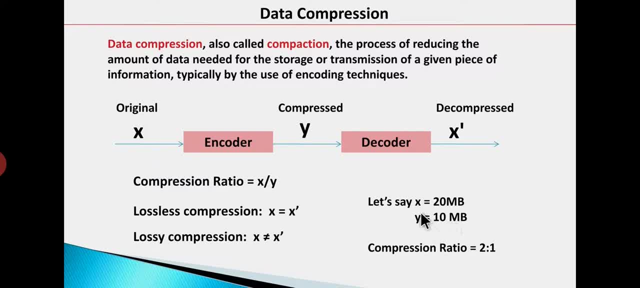 y becomes 10 MB, So compression ratio becomes x by y, which means 2 to 1.. Okay, So that means the more memory is required for x, the more compression ratio is required for x. So its half of the memory will be required to store Y. so what will happen? your memory is being saved. 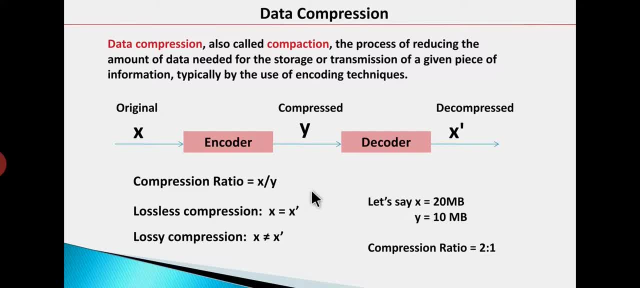 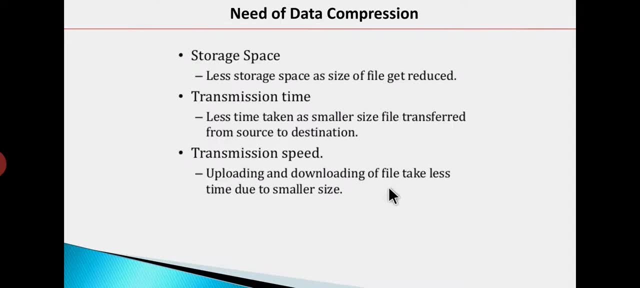 Okay. so to measure how much compression is achieved, we use compression ratio. Okay, now what is the need of data compression? So there are three advantages. one first is storage space. next, storage space. as file size of file get reduced means the storage of data. 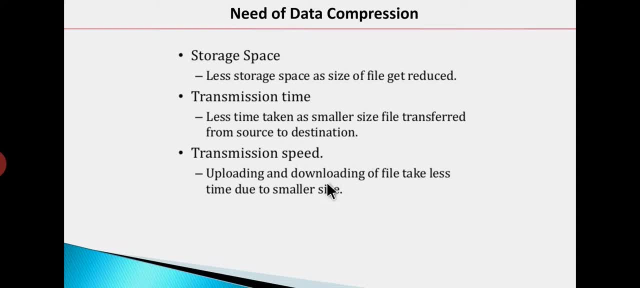 has reduced. we have seen this is 20 GB file, mb file. after compression it becomes 10 mb. So by the memory of 20 mb, 30 mb compression data is stored in half the memory. so our storage is being saved. So we use data compression for next storage. 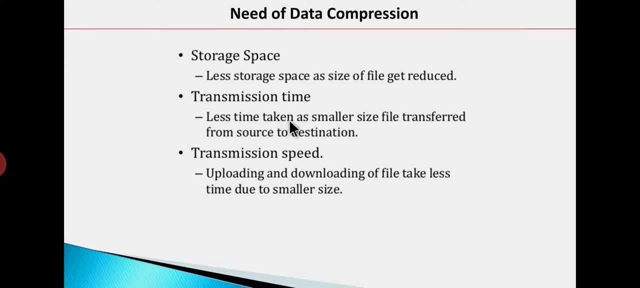 Second is transpose. You see, this is in différence with on job. we use on job using transpose bothITY. and also we have the 파 Д, which is not flat data, But that is because it is its function, Next time taken as smaller size file transferred from source to destination. 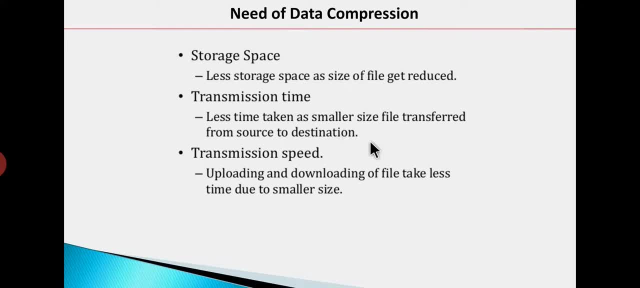 If you want to transmit a file from one device to another device, then the smaller the size of the file, the faster it will be transmitted. So in actual, we do not transmit original data, but we transmit compressed data because its size is less than original data, So the transmission time becomes smaller. 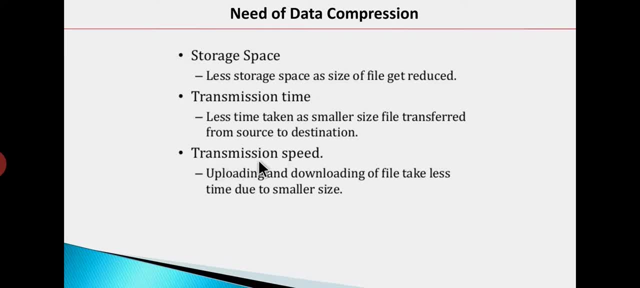 The third one is transmission speed. Uploading and downloading of file take less time due to smaller size, So transmission speed increases. If you are uploading or downloading a file, then if the size of the file is small then it will be uploaded and downloaded faster. 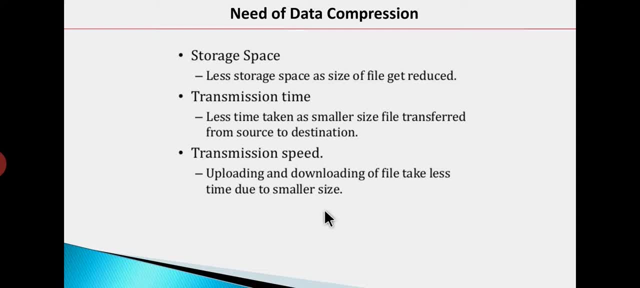 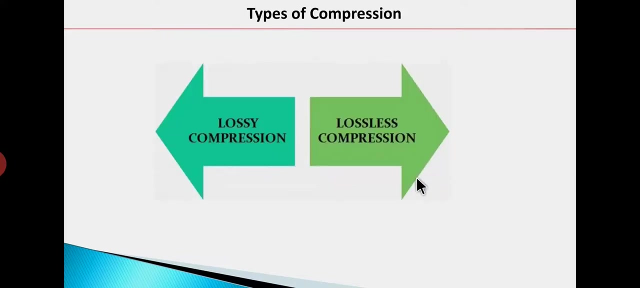 So in actual, when we upload and download, that is the compressed file, not the original file. So the compressed file will take less time with high transmission speed while downloading and uploading. So these are the three major advantages for which we perform data compression. Let's see the types of 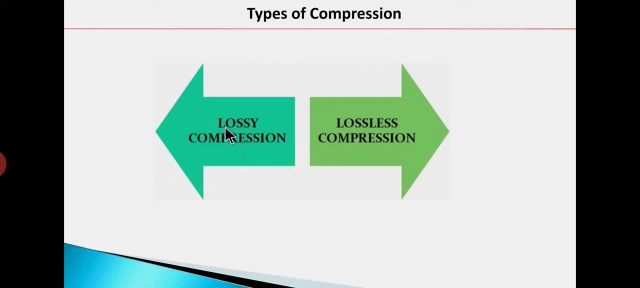 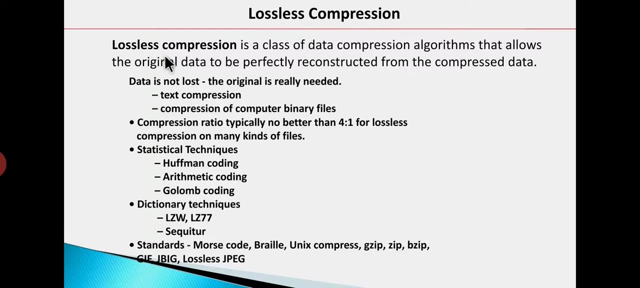 compressions. There are two types of compression. One is nausea compression and other is nauseousness compression. Let's see one by one. First, we see nauseousness compression. So nauseousness compression is a class of data compression algorithms that allows the original data to be perfectly reconstructed from the compressed data. 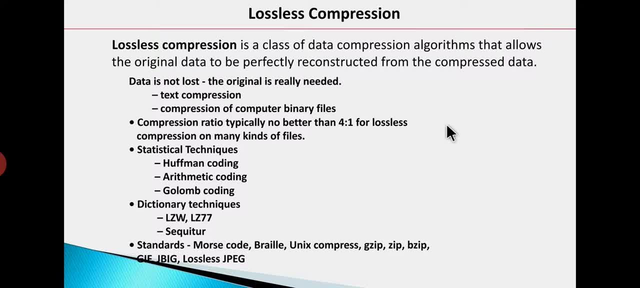 So we saw that in nauseousness compression there is no loss of data. The original data is when we compress. After compressing, when we decompress, we again get the original data. So x is same as x dash. It means there is no loss of data while decompression. This is what is called nauseousness compression. 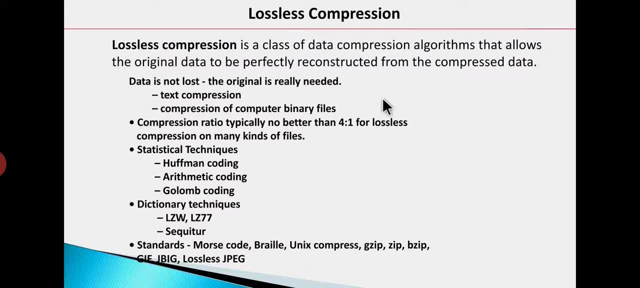 There are many scenarios where we cannot tolerate the loss of data. For example, if we are sending a text file and there is a sentence in it and even if one character of that sentence changes, the meaning of that sentence can only change. So the text files we send. we don't want there to be any loss of data. 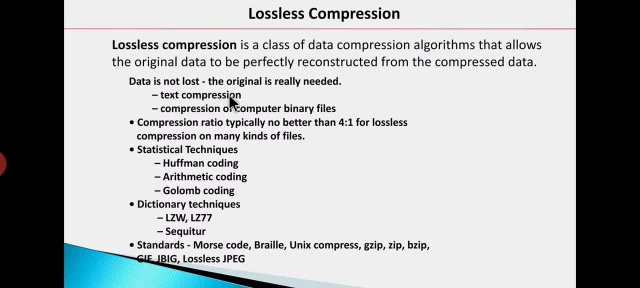 So text compression, basically all the text compression techniques, come under nauseousness compression, Because if there is a sentence in English in which one or two words change, or even if one or two alphabets change, then it is possible that the meaning of the whole sentence changes. 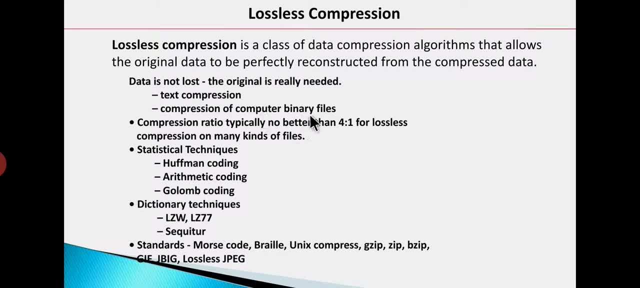 Or there are such things like compression of binary files. It means there is a software whose exe file is in binary form. For example, when we install the software, we get an exe file. Now you compressed the exe file and you transmitted it. 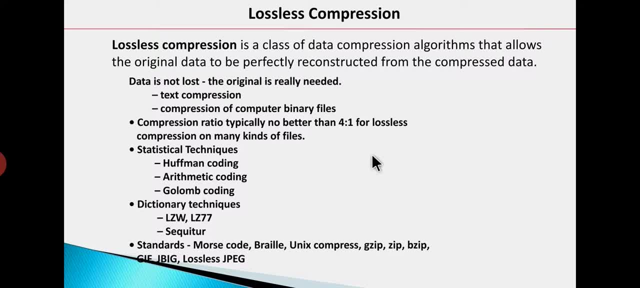 Or you decompressed it later and you will not get the original file, Then that software will not be able to be installed. So if there is a binary file, then if you have any 0 of 1 or 1 of 0 in it, 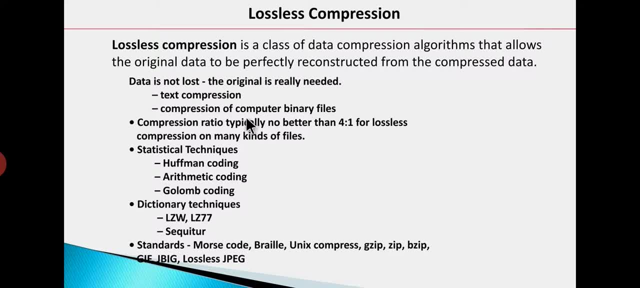 then the whole meaning will change. So that's why, if there are binary files, if we are doing their compression, then we will want that compression to be nauseousness compression. There are many images in which we use nauseousness compression, For example, if there is an x-ray report. 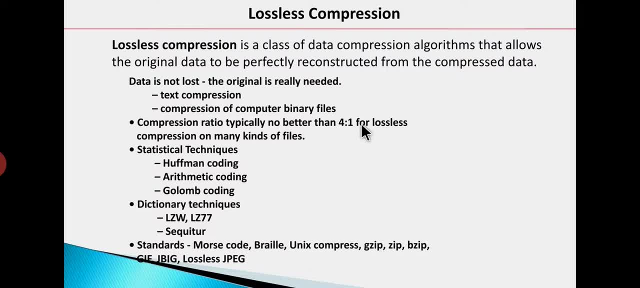 there is an image of an x-ray and after decompressing it there is some loss of data in it, then it will be difficult to diagnose the doctor. So if the x-ray is fine, the image of the x-ray, we will want that when it is decompressed. 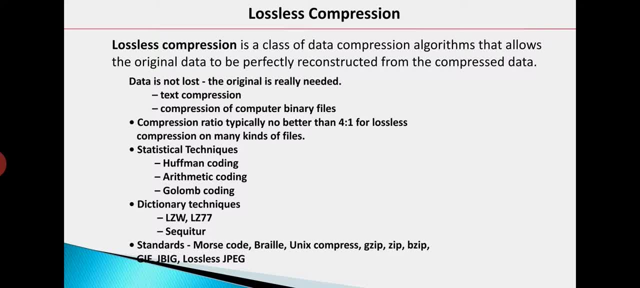 then we get the original image. Otherwise, if there is some loss of data in it, then the doctor will not be able to diagnose. Okay, so this is So. in such a place where we cannot tolerate the loss of data, there can be a loss. 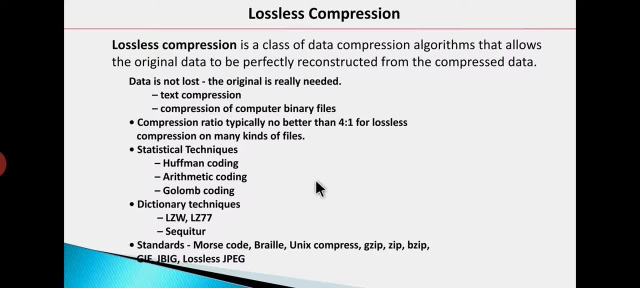 In that place, we use nauseousness compression techniques. Okay, The compression ratio is typically no better than 4 is to 1 for nauseousness, So the compression ratio will not be more than this. What does 4 is to 1 mean? 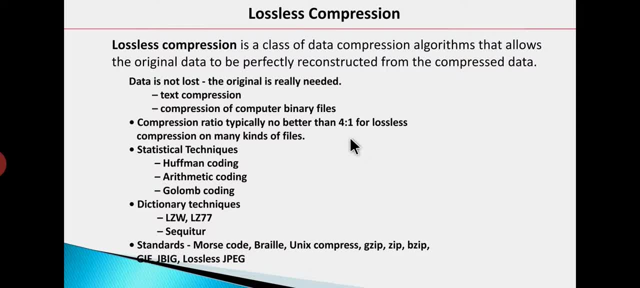 You will not be able to achieve more than 1 fourth compression. Okay, And the techniques used in nauseousness compression means the nauseousness compression algorithm, the techniques we use for it. basically the important techniques are Huffman coding, arithmetic coding and Goon number coding. 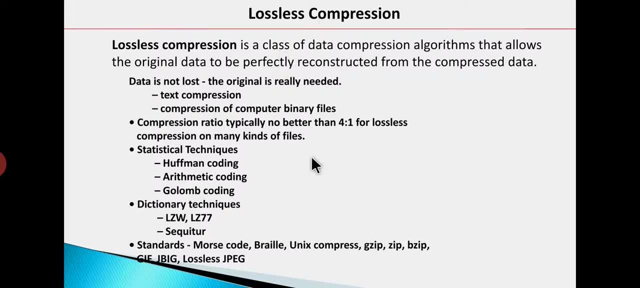 These techniques are used for nauseousness: compression algorithms. Okay, There are some dictionary techniques which are adopted in alphabets and text files. They are NZW or NZ77 or Suiketer. Okay, And some standards have been made. 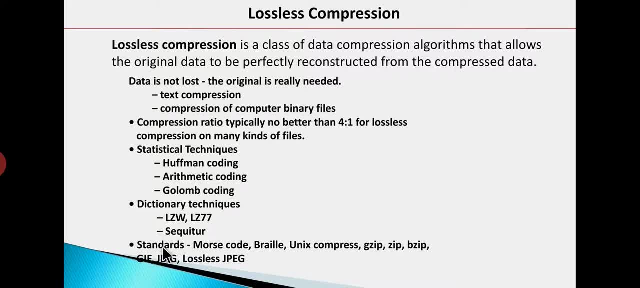 which have been made, which every manufacturer, every data compression software that is made follows them, Like: there is Morse code, brain the blind people have brain NIPI, they have standards. There is UNIX compress, there is GZIP, you know ZIP file. 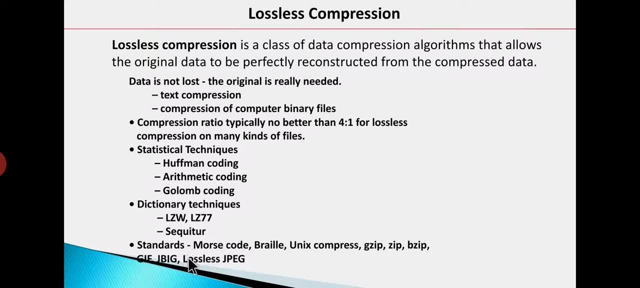 Okay, There is binary ZIP. This is called nauseousness JPG. So JPG comes in two forms: nauseousness and nauseousness. Where we cannot bear the nauseousness in the image, we use nauseousness JPG Otherwise. 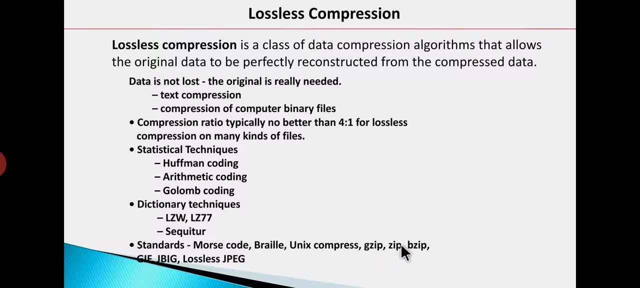 we use nauseous JPG, So these are the standards. Whenever you see this ZIP file, understand that the technique used in it is nauseousness compression technique. Okay, So this is what Nauseousness compression. Its position is nauseousness compression. 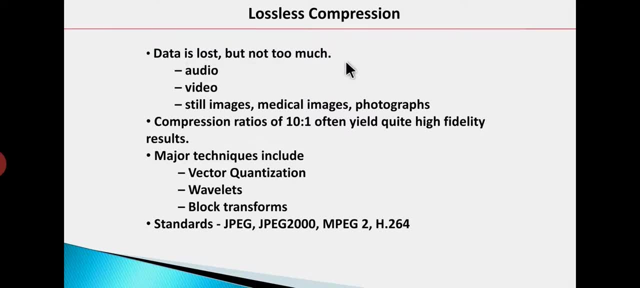 Data is nauseous, but not too much. Data is nauseous. X is not same as X dash, But it does not get so much nauseousness that the whole data gets spoiled. Okay, It will be as much nauseousness as we can bear it. 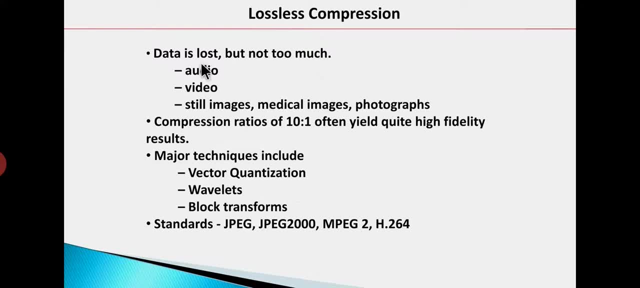 Okay. We generally use this kind of technique in audio video file or in some images or photographs Like audio, some song: Okay When you are listening to it by decompressing after decompression, when you get the file. 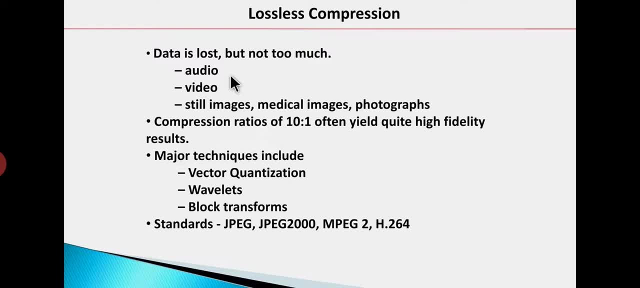 you are listening to it. So if the audio gets a little bit here and there, then you will understand the whole song. Okay, There will be some difficulty, but the song is understood completely. Same way if you are watching a movie. 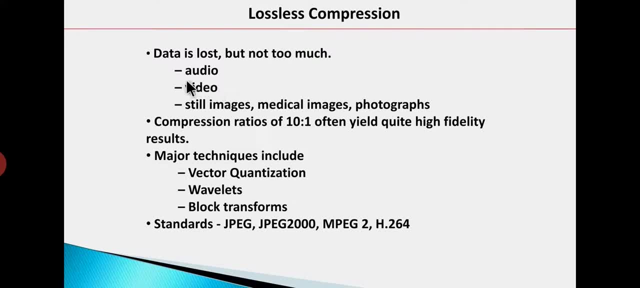 then it is a very big file, video file. So if in one or two frames it is happening here and there there is no clarity, then you will understand by looking at the previous sequence what is actually happening in this frame. So where there is not much difficulty. 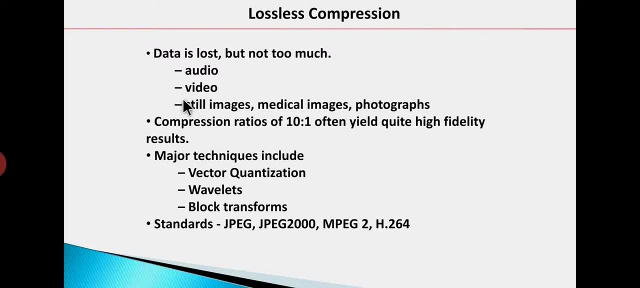 where we can bear a little bit of nauseousness, we use nauseousness, sorry, nauseous compression- Here. by mistake nauseousness is written. this is nauseous compression. Okay, So compression ratio is 10 to 1,. 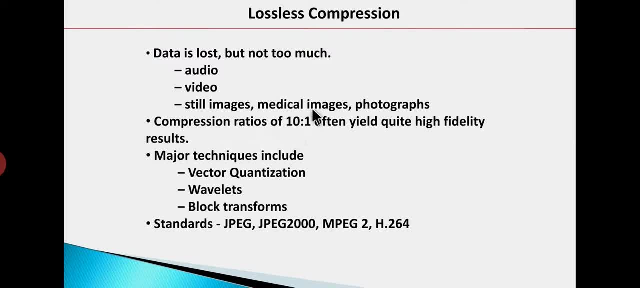 often in good, high to dainty regions. So here, nauseous compression. in nauseous compression the compression is very high as compared to nauseousness. You can reduce the size by 10 times. The size can be reduced by 10 times. 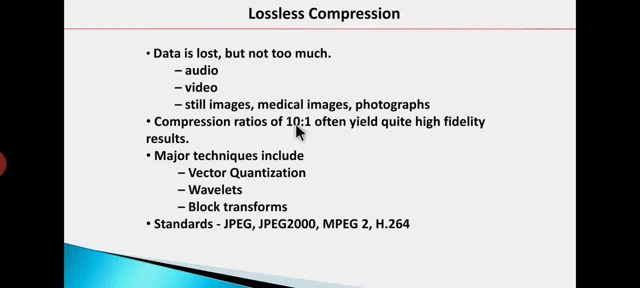 There it can be reduced by 4 times. Because what is in the nauseousness? there is a restriction that data should not be nauseous in any case. This restriction is removed here. Okay, The techniques generally used in nauseous compression: 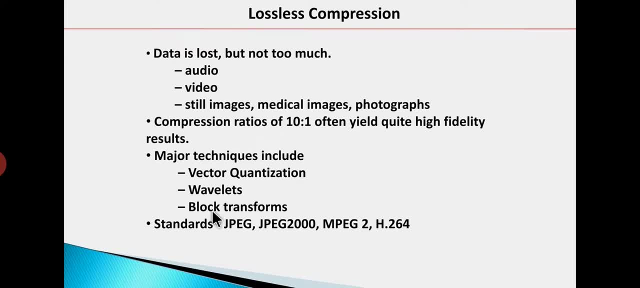 that is, vector quantization wavenets and block transforms. Okay, And the standards for this are JPG images which you normally use to store images: JPG 2000,, MPG 2, H.264.. So these standards, these standards come under nauseous compression. 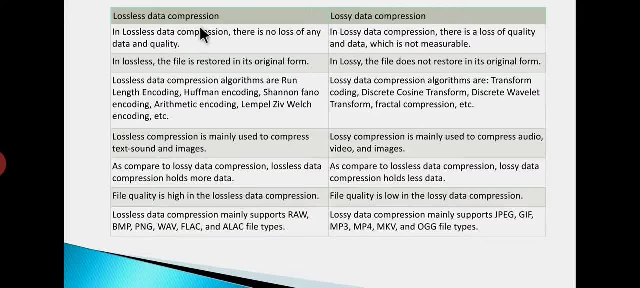 Okay, Now this is the difference between nauseousness and nauseousness. So in nauseousness- data compression- there is no loss of any data and quality. So we know that in nauseousness, there is no loss of data and the quality is maintained. 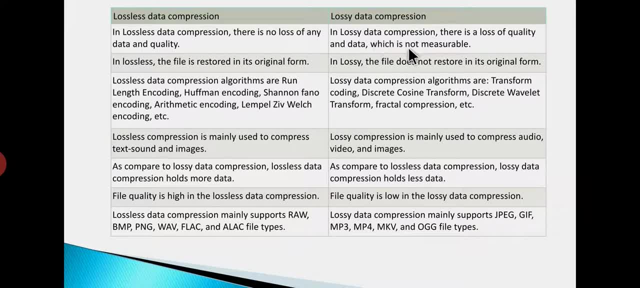 And in nauseousness there is a loss of quality and data which is not measurable. Okay, So here there is some loss of data as well as quality In nauseousness. the file is restored in original form. Okay. 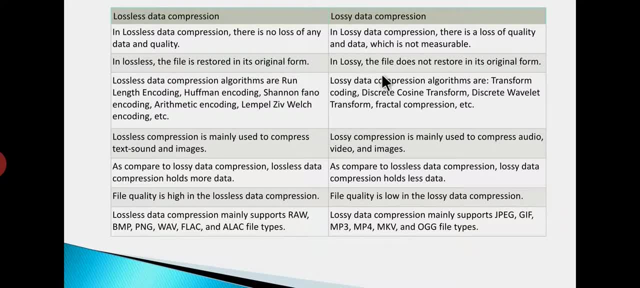 In nauseousness you get the original form again And in this there is a loss, So you cannot restore the original file. Okay, Nauseousness. data compression algorithms, are they have some names run length encoding: Huffman. 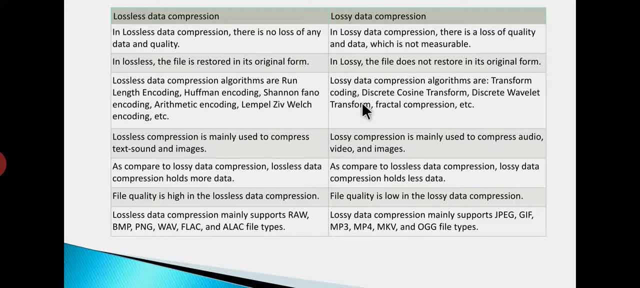 all these techniques are used For what? For nauseousness, data compression And techniques used in nauseousness data compression are: transform, coding, discrete cosine, transform discrete webnets, etc. These are the techniques used in nauseousness and nauseousness data compression. 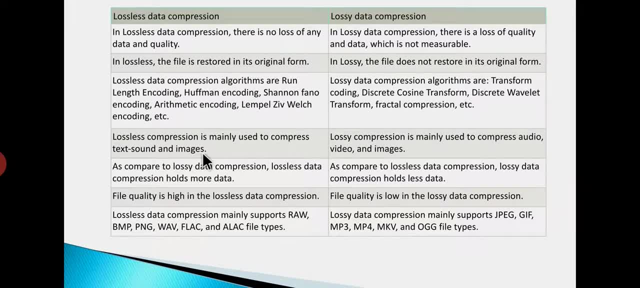 Nauseousness compression is mainly used to compress text, sound and images. Many nauseousness compressions are used to compress text files, sound files and images. Okay, And here we use Nauseousness data compression in audio. 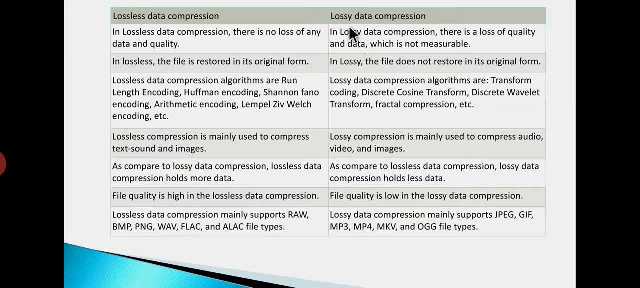 video and images. Both images are in audio. In audio and video, mostly we use nauseousness compression. As compared to nauseousness compression, Nauseousness data compression holds more data. That means the size of compression increases as compared to nauseousness. 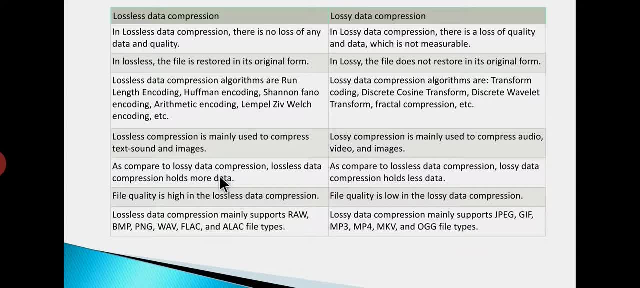 You can reduce the size more in nauseousness And the size in nauseousness does not reduce as much as compared to nauseousness. Okay, the file quality is high. it is obvious there is a complete nauseousness. file quality is low due to nausea and these are some of the standards, like BMP, PNG you. 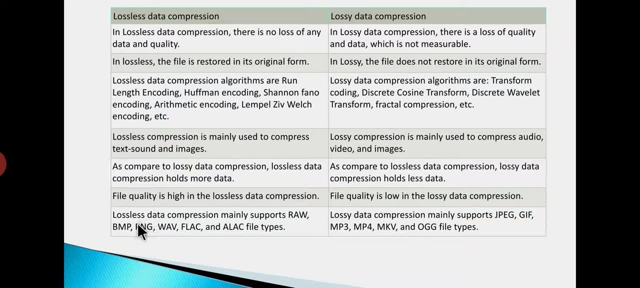 know PNG file. PNG is used for image files, so PNG- is this standard- comes under nauseous data compression, or MPV4, which we generally use for video, or MP3 for audio files, these which are commonly used. these are the compression techniques that come under nausea data compression. 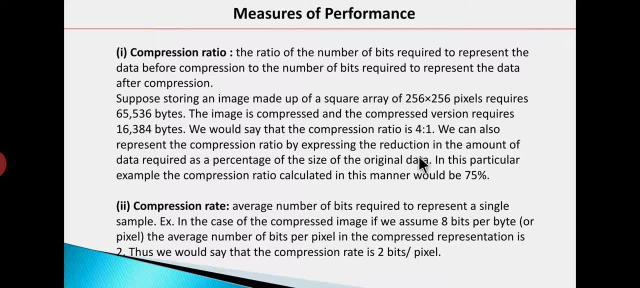 Now comes the measures of performance. if there is any technique, if there is a compression technique, then how will we measure its performance? so it has some parameters. mainly these are two parameters. one is compression ratio, that how much compression is being done in. 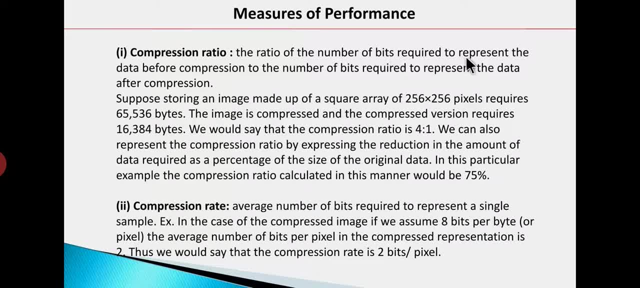 file, the ratio of the number of bits required to represent the data before compression to the number of bits required to represent the data after compression. so what is this ratio that I saw there? x by y. what is x? So what is x? 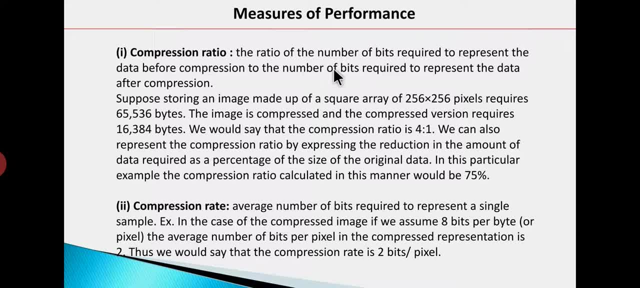 This is the original file size and y is the file size after compression. the ratio of these means that how many bits were in the original file and how many bits of the file is being stopped after compression. the ratio is the compression ratio. Suppose that an image is fine and the square array means that the size of the window on 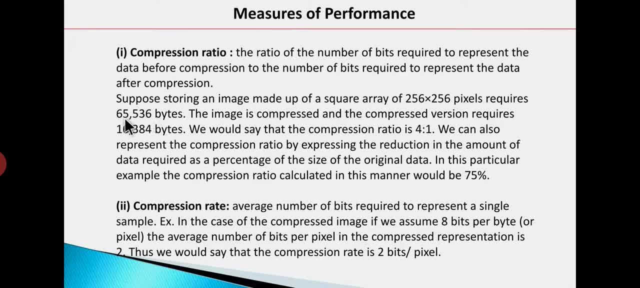 which the display is being displayed is 256 by 256 pixels, 65,536 bytes. the image is compressed and the compressed version requires 16,384 bytes, So the compression ratio will be 65,536 by 16,3xy. 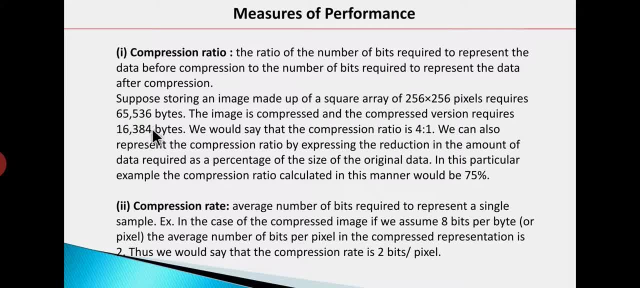 There is an x, and this is the original file, and here is the y, so both: the x is by y and it comes out to 4, is to 1.. That means that the size is reduced 4 times. Okay ratio by reduction in the amount, which is 75%. either you can tell in ratio or in percentage. 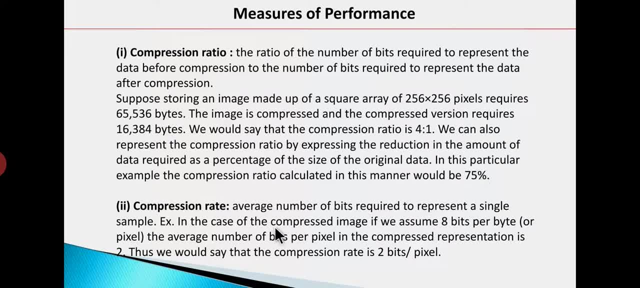 that how much percentage size is reduced? that is 75%. Second parameter is compression rate. what is compression rate? average number of bits required to represent a single sample. to store one sample, how many bits are required on an average? suppose 8 bits per byte and pixel is in original file and after compression. 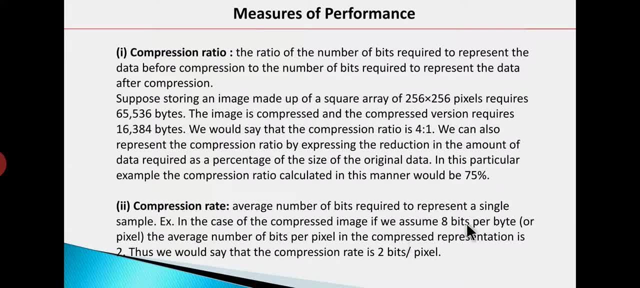 it becomes 2, means in original file, to store one pixel we need 8 bits, and after compression it becomes 2.. Now what will happen? 2 bits per pixel means before compression we need 8 bits in one pixel and after compression we need only 2 bits in one pixel. so here the sample is a pixel. 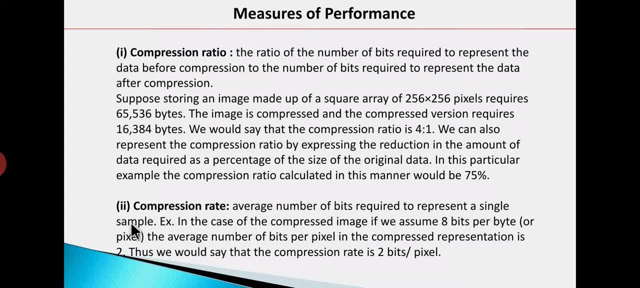 so here we have to find out the compression rate, that how many bits are required to store one sample in original file, and after compression, how many bits are required to store the same sample. this is what compression rate. The third one is fidelity and quality. 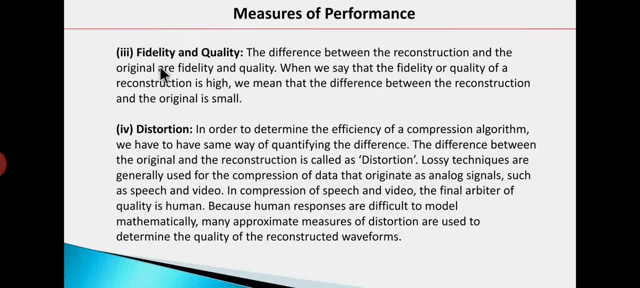 The difference between fidelity and quality is that the difference between fidelity and quality is the difference between reality and not, And our main question, The difference, ie the difference between theётся difference you can find by Its usually and I case when we have sales. 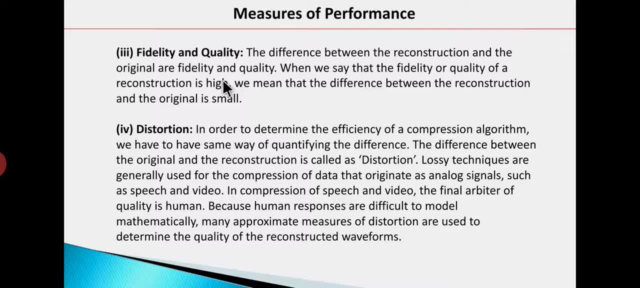 requirements for data and execution. So files Are there. Yes, So when we say that fidelity or quality of a reconstruction is high, we mean that the difference between a reconstruction and the original is small. So this parameter is applied only on lossy compression. 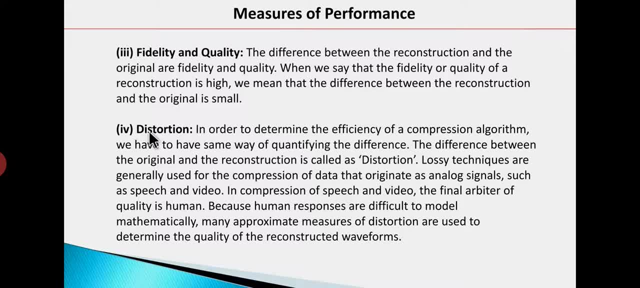 And the next one is distortion. This is generally used in video files where audio is used in order to determine the efficiency of a compression, So this parameter is applied only on lossy compression. And the next one is distortion. This is generally used in video files where audio is used in order to determine the efficiency. 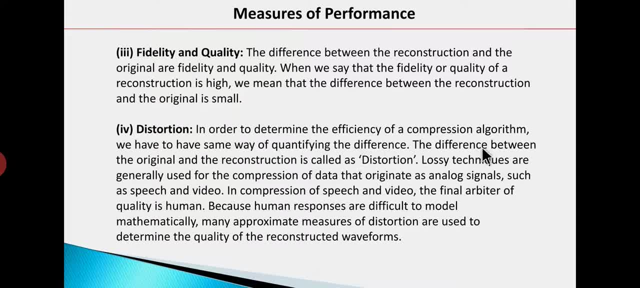 of a compression, We have to have somewhere quantifying the difference. The difference between the original and reconstruction is called distortion. I mean the difference between the original and reconstruction is called distortion. This is also applied on lossy techniques Because in this data loss and happen will differ between each other. 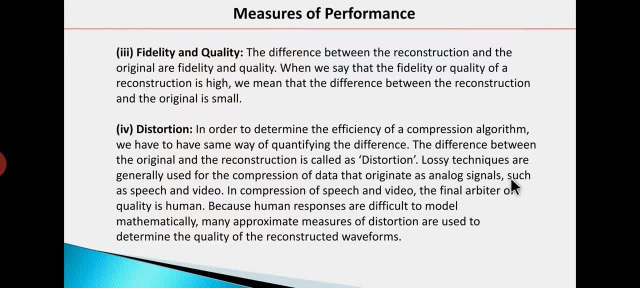 Like an aux signal is used instead of audio. So this is the difference between the original and reconstruction, Because in this data loss and happen will differ between each other, such as speech and video. we are using ANOX signals, So if we are compressing video and audio, 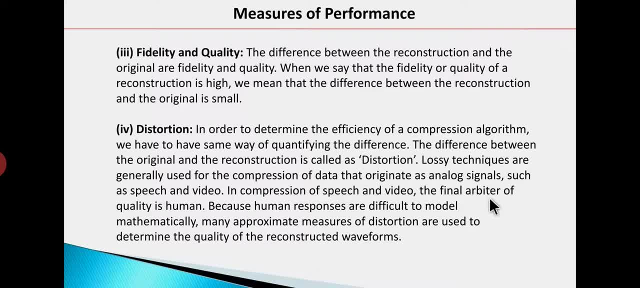 then how much has the quality degraded? Who will tell this? The person who is listening to it. For example, there are two people and you give them the same song to listen to or give them the same video to watch, And there is some nausea technique used in it. 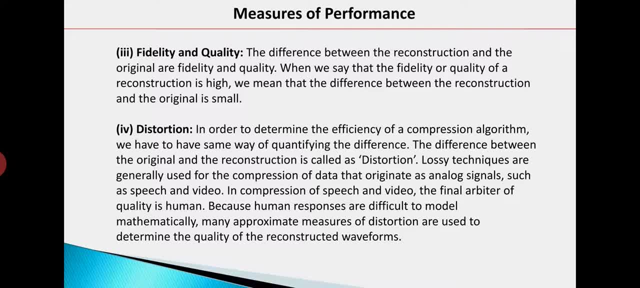 Generally there is nausea. So one can say that there is not much difference. One can say that there is more difference. One can decide how much distortion has happened. So it is very difficult to say how much distortion has happened. It is very difficult to say this. 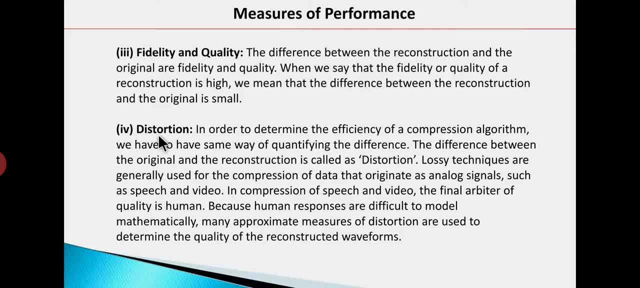 because the person to person will differ. Someone will feel that the distortion has decreased. the quality is a little less. someone will feel that the quality has fallen more. Because human resources responses are difficult to model mathematically, many approximate measures of distortion are used. 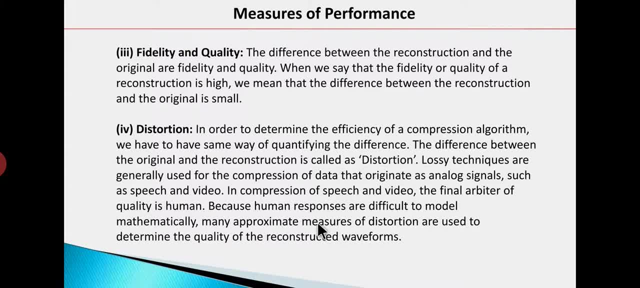 to define the quality of the constructed waveforms. So this distortion is also used. I said in the audio-video where the audio is earlier clear, then a little bit of clarity has been reduced. You say that so much clarity has been reduced. 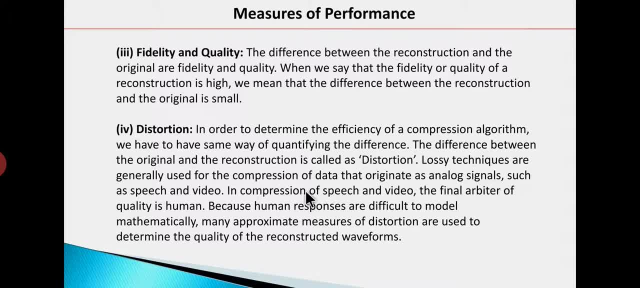 If there is more, then there is more distortion. If there is less clarity, then there is less distortion. The same is with the video. So we actually use this in nausea. We do not use it in nauseousness because audio-video compression techniques.